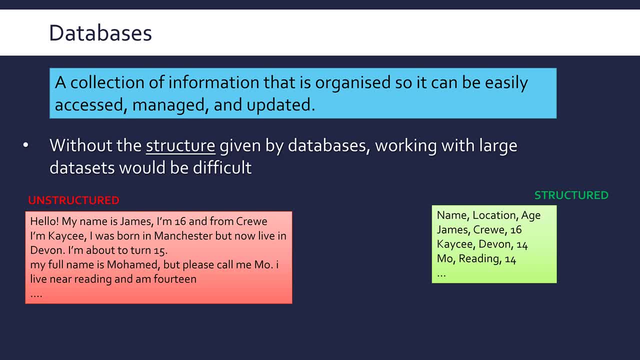 having that structure is so much more preferable. so this might be a snippet from a text file like a CSV file, where you've got the names, location and age in a much more structured format. so we've got sort of a header, row, name, location, age, and each bit of data is separated by a comma. this is called a CSV file, and 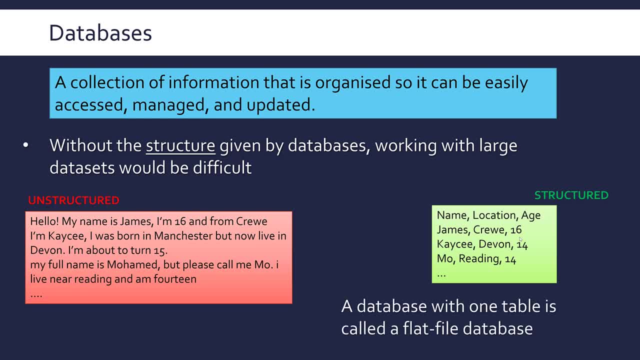 this is really a database- not maybe what we imagine with a database, but this is a really simple database. because it's a really simple database? because it's a. in effect, we've got a table here, we've got columns and we've got rows. now, a database with only one table is called a flat file database, and they're not. 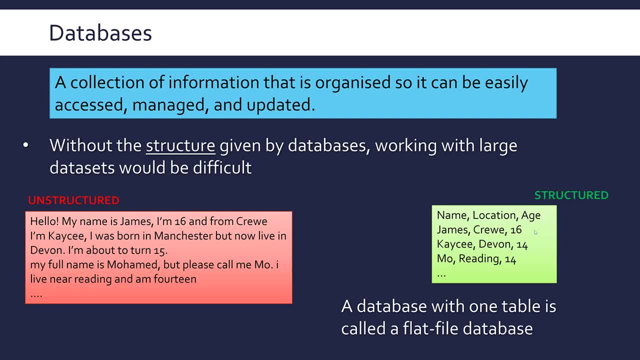 really so useful. they don't scale very well when you have lots and lots of data. but to introduce two important words: records and fields: records are really our rows in the database and the fields are really our columns. so when you talk about databases, think record for row, think 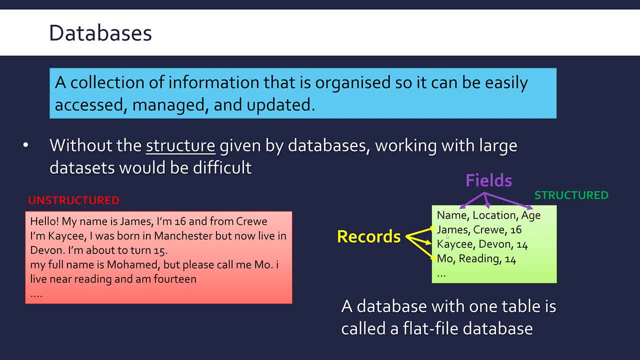 field for column. so you know, the record for James has got three fields, James Cruz 16. the record for Moe has got Moe reading and 14 as those fields. so the intersection of a field and a record is the actual individual bit of data. and if 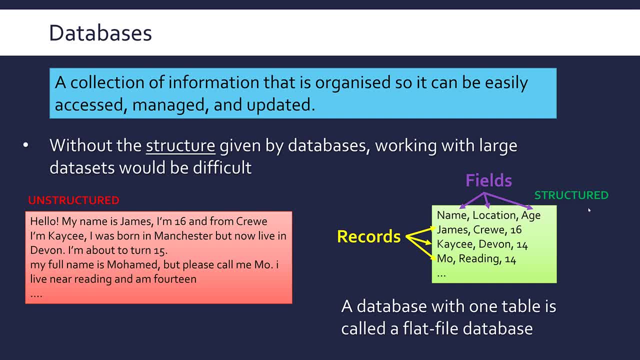 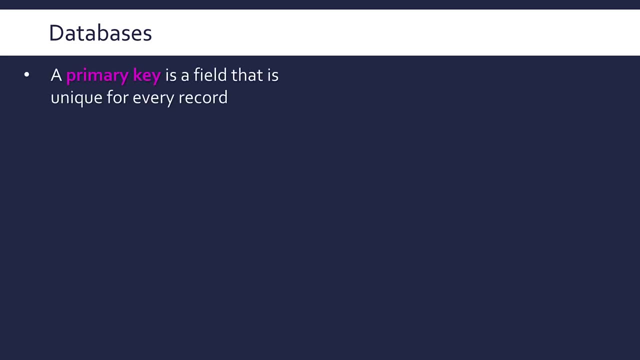 we can see why having a structure makes it much easier. you could, without too much difficulty, write some code which can interpret this database, not the text on the left, but we can get better than a flat file database. before we do, let's just mention another key bit of terminology, which is primary key, so a. 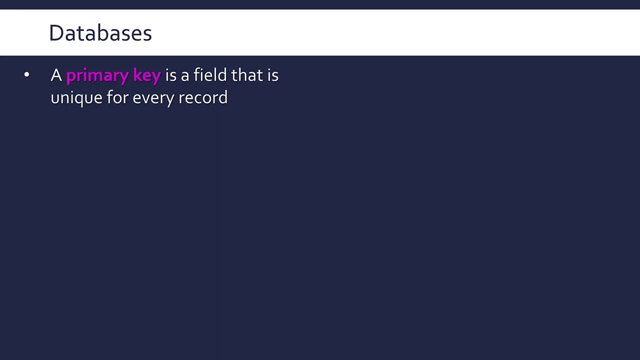 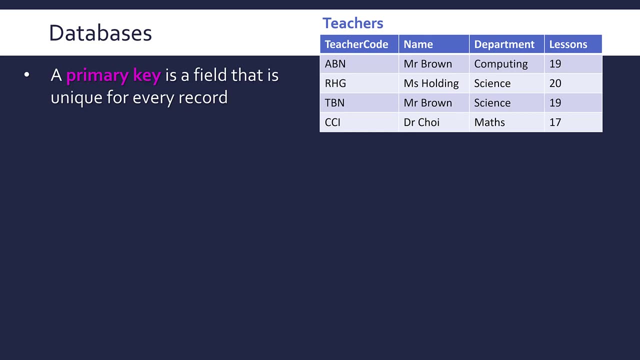 primary key in database, lingo is a field that is unique for every record in that table. so here is a table- an actual table this time- of teachers and their names, departments and lessons. usually if you see a table in an exam, you'll see, obviously you'll see a table in the database and you see how many tables you're seeing. 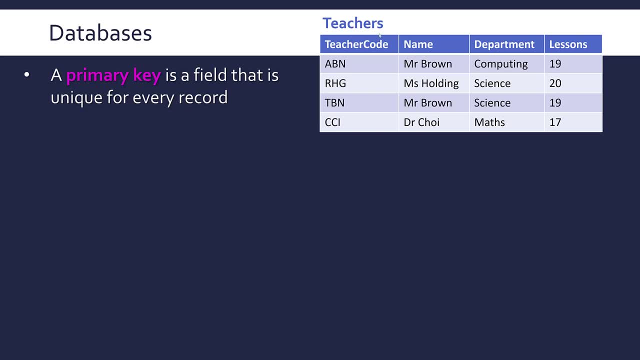 headings, obvious records, but usually there will be a name, often plural, capitalized, etc. The fields should really be one word, or the field names, at least, should be really one word. In terms of this table, what field is unique for every record? Well, only one, that is, teacher code. So if you are making a formal database, you need 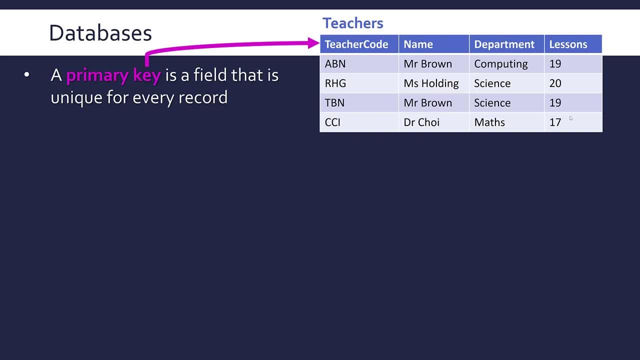 to make sure you have a primary key for every table. You must have a unique field, otherwise you can't uniquely identify a record. Here we've got two Mr Browns. downside of having a common surname: Without the teacher code you wouldn't be able to distinguish between the two. One is science, one is computing. but how would? 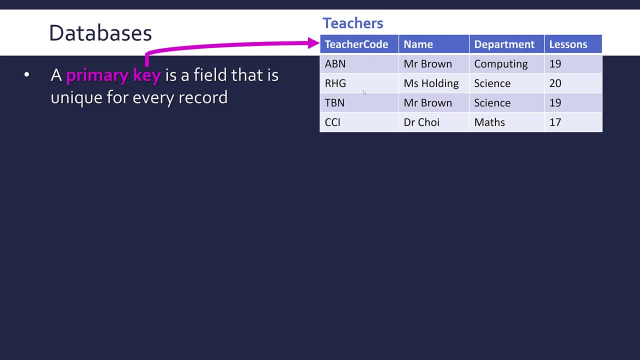 you know if you had no other information, Whereas if you have a teacher code, it narrows it down to just one record. So this is important when we start to want to search a database or change a database- It doesn't matter what it is it. 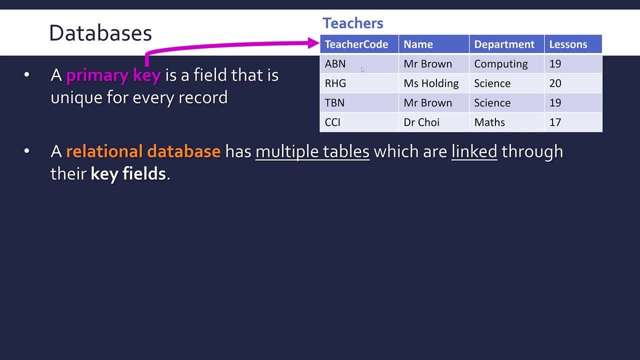 can be a number, can be a code, in this case, often an IE. So watch out for these. you need to have one in every table. Now, if a slightly better database compared to a flat file database, is a relational database which has multiple tables which are connected, They're connected, linked through their. 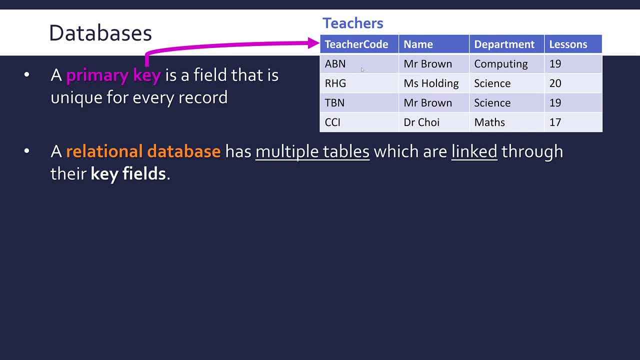 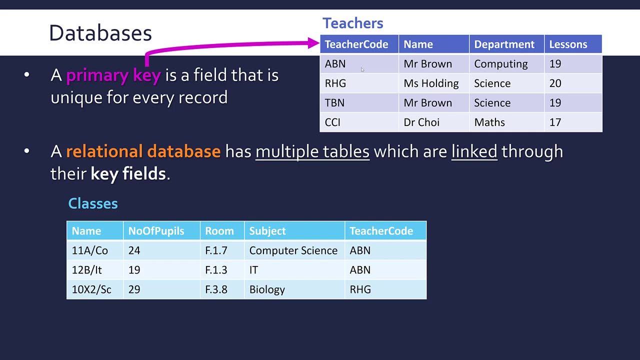 key fields. So primary key is useful and needed to access each individual record, but also it enables you to connect up similar but different tables. So let's say we've got another table related to schools which has different classes, So the class name, how many pupils there are, the room, etc. etc. 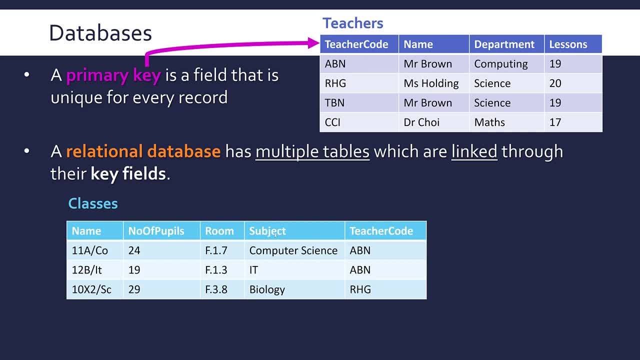 Now these two tables are connected through a key field. The primary key for classes is most likely going to be the name of the class, or the class code, I guess you could say, because it wouldn't make sense to have more than one class with the same name. Now the rooms and number of pupils and subjects are unique. 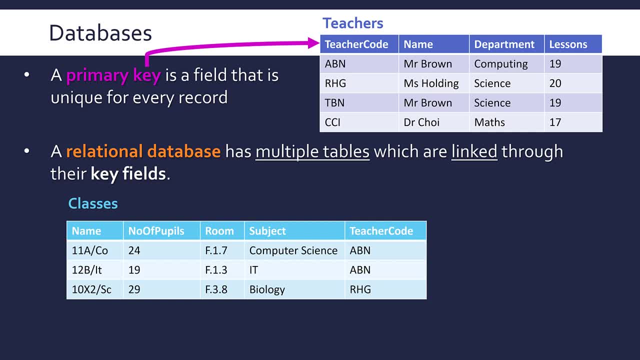 but it would be more sensible if the name of the class was the same as the class code. But also: look, we've got teacher code Now teacher code is another key field, but a different type of key. This is a foreign key. So a foreign key is a field in one. 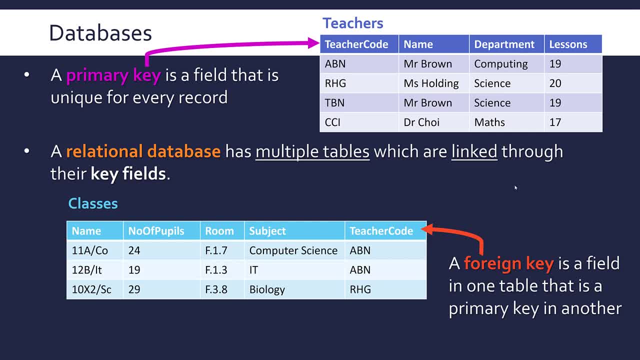 table that is a primary key in another table. So teacher code is primary in the teachers table but because it's also in classes, it's therefore a foreign key. Subject room number of pupils are not foreign keys Because they're not primary keys in another table And name isn't foreign. 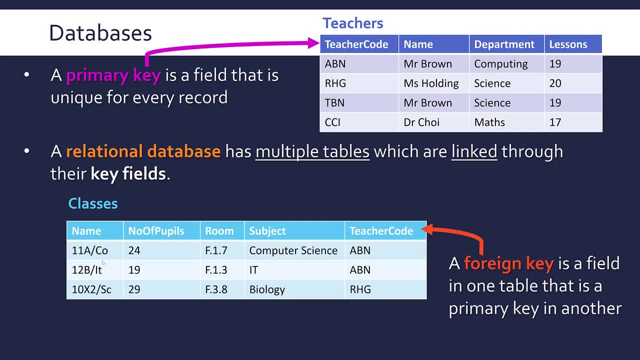 because, again, it's not a key in another table and its primary key for this table. So having a foreign key enables you to connect up these two tables. because if I'm looking at 11A Co a year 11 computer science class, I can see ABN is 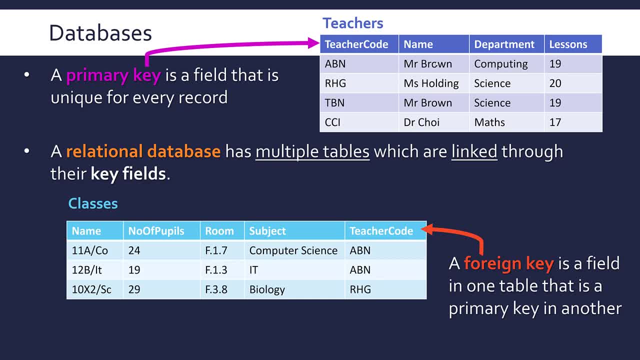 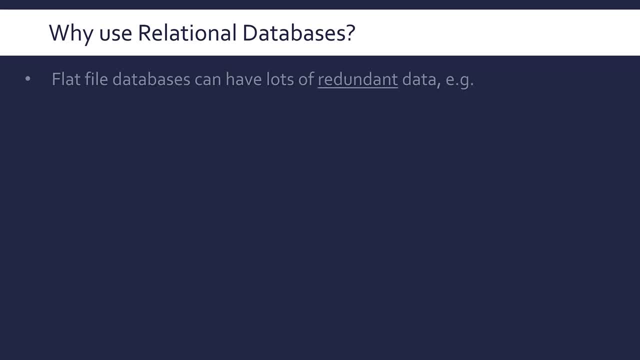 the teacher, and so I can look up ABN in the other table Enables you to connect them together. Now this all begs the question why? Why not just keep databases really simple as one table with all of your data in it? Well, flat file databases can lead to you having 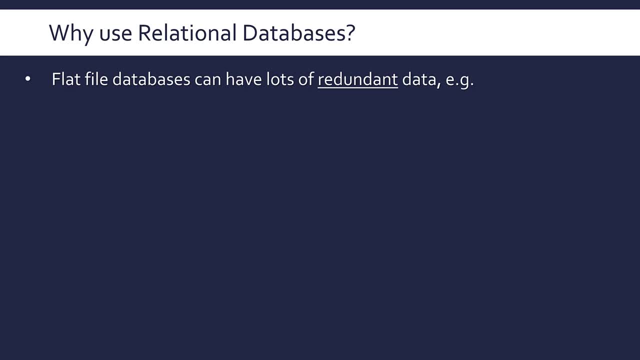 lots of redundant data. When things are redundant, you've got more of it than you need. If somebody's made redundant, they lose their job because they're not needed by the company anymore, and redundancy can be good in certain areas of computing. You might have a redundant server as a backup, but in databases it's. 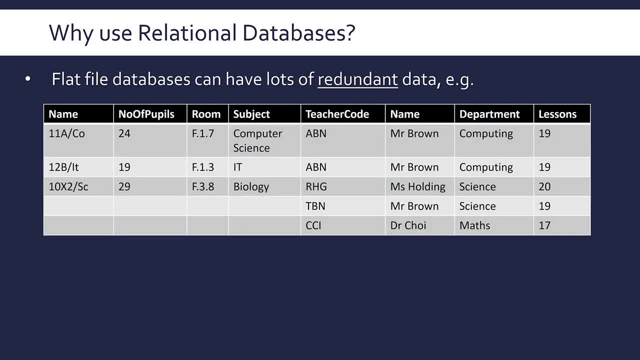 not good because you have wasted storage space. So here I've got both tables combined into one big table, so a flat file database here and we have some redundancy. The redundancy is in this top right area where, because ABN is teaching two classes, the data for him is repeated twice, which is just not. 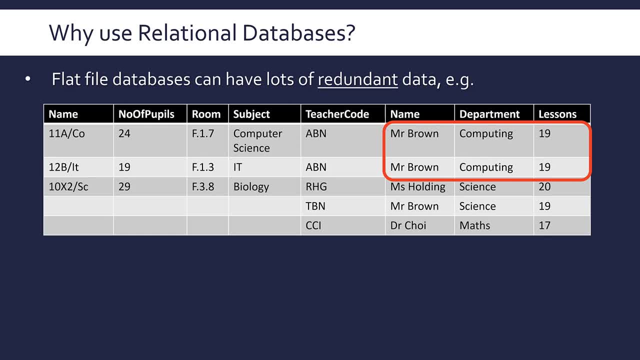 efficient. I don't need to repeat it twice. I could keep it once. So that's the redundancy. Now the code ABN is repeated twice, but you have to have some repeats because that's how they connect up the tables. Teacher code would be a foreign key if these were two. 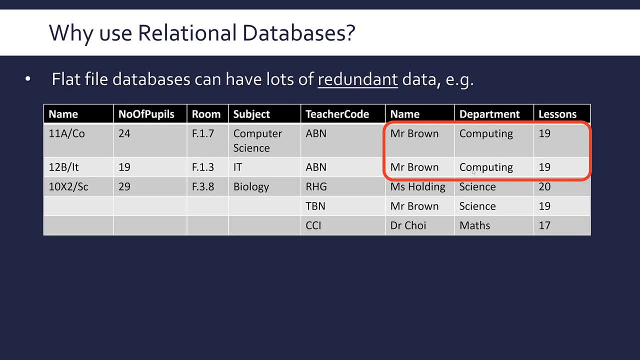 distinct tables, But that's wasteful. Now, if that was all 19 classes, all 19 lessons, that becomes especially wasteful. Now we've also got a gap in the bottom left where certain fields are empty for our bottom two records. Maybe we haven't got. 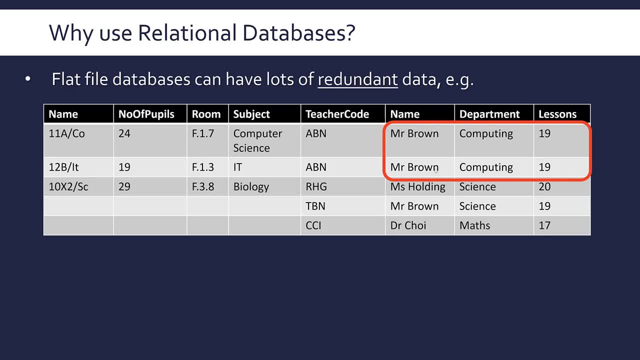 assigned a class yet That is wasteful too, but not quite in the same way. We've got a gap in the bottom left where certain fields are empty for our bottom two records. Maybe we haven't got assigned a class yet. That is wasteful too, but not quite in the same way. 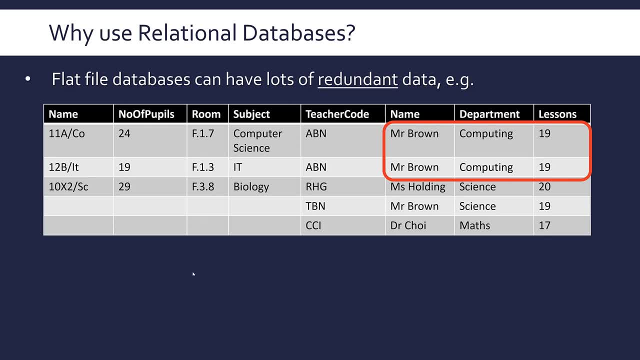 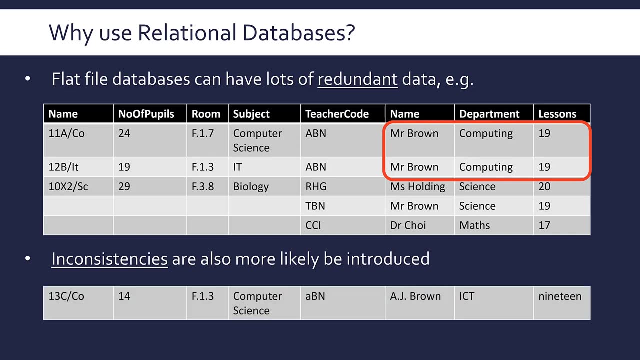 Right, that could be redundant if add lots of it and there were loads more gaps, but it's just not efficient. But that's our main problem: it's really wasteful And it can also lead to more errors, in particular inconsistencies, If you are adding more data to it and you're having to fill in more fields than are really.